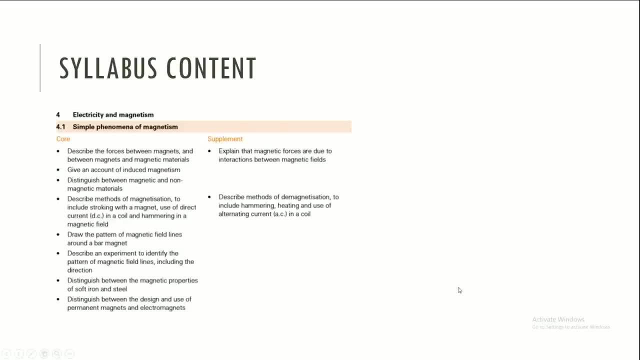 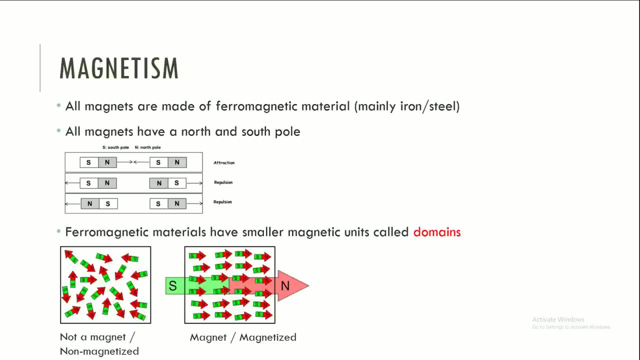 read through, and we will begin shortly. So magnetism: Well, magnetism, of course, has something to do with magnets, So magnets are made of ferromagnetic material. The main things that you will come across in your course would be iron and steel, And all magnets have a north and south pole, and these poles 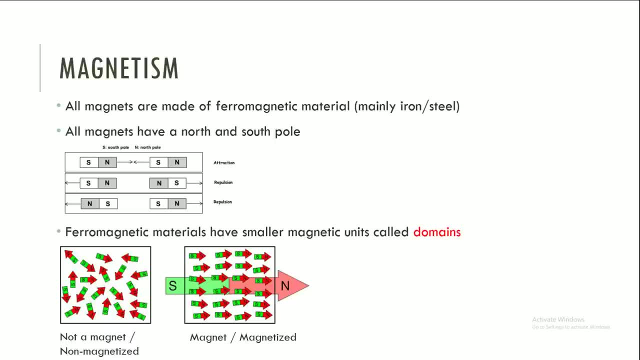 can either attract or repel, depending on the interaction. Now, when you have opposite poles, for example a north and a south pole, they will always attract. If you have two same poles or like poles, they will always repel. So opposites attract and same poles. 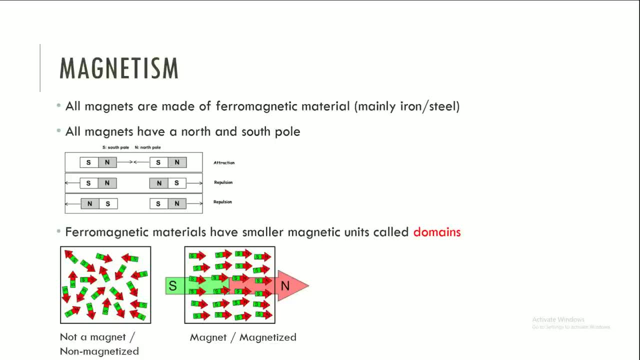 repel. That's a very, very important concept, And so ferromagnetic materials, which of course are what magnets are made of, are special because they have smaller magnetic units within them, called domains, And these little magnets or magnet units called domains. 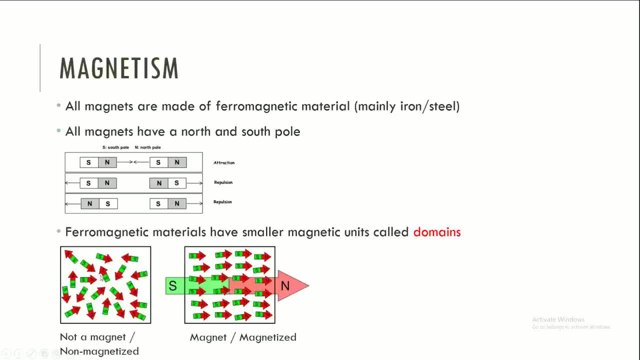 each have a north and south pole as well, And that is sort of the easiest way to sort of demonstrate this idea Now in a non-magnetized ferromagnetic material, for example iron. so just because something is ferromagnetic doesn't mean that it is automatically a magnet. 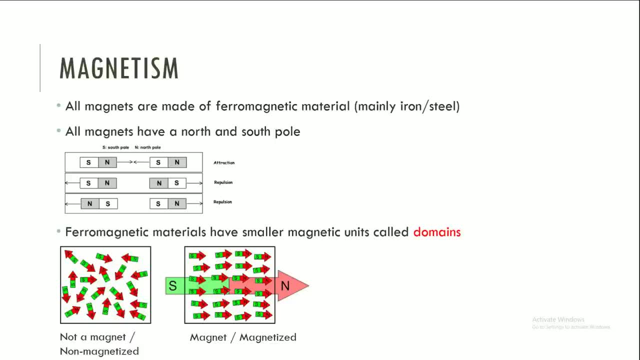 If something is a magnet, then it has to be a ferromagnetic material. Do you see what I mean? And so in a non-magnetized piece of iron, which is of course ferromagnetic, you've got these little domain magnets inside the iron that are randomized in orientation. They're 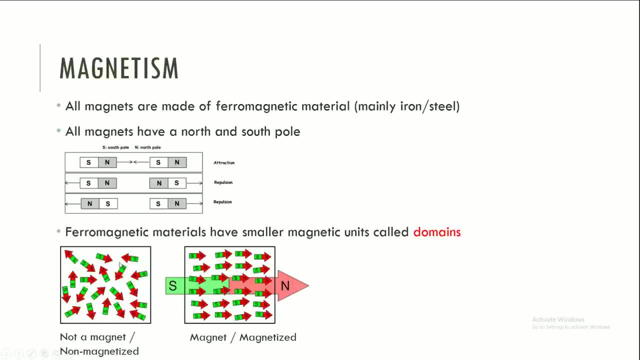 sort of facing all over the place and they don't really have any sort of unified direction. And that is essentially why the iron is not a magnet, but it is ferromagnetic, suggesting that it has a potential to become magnet. And we'll talk about induced magnetism later, but for now just understand that in. 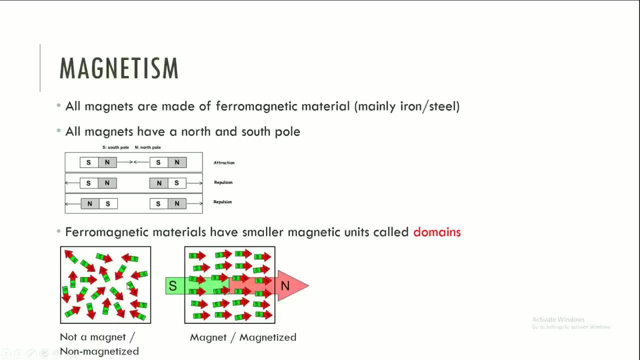 a non-magnetized magnetic material, the domains or the little magnetic units inside of them are basically randomized in orientation. Now in a permanent magnet you have these domains that are all unified in a particular direction And, as you can see in this right diagram here, all the little domains have their north. 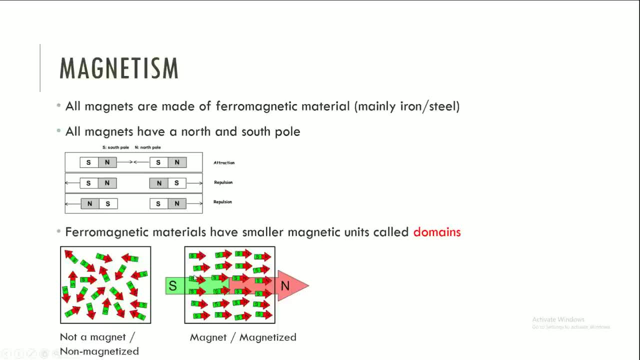 poles facing a certain direction and the south poles facing the opposite direction. And therefore, if you sort of combine that all in together and you look at the bigger picture, you see that the left side here is basically the south pole of the entire magnet and the right side 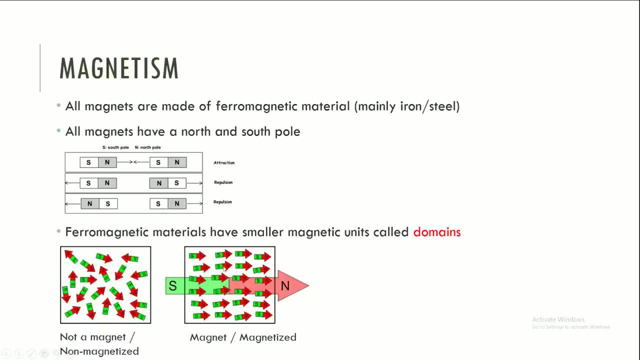 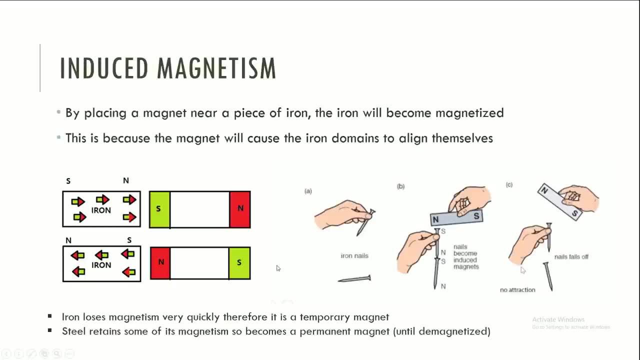 here is the north pole, and that is all dictated by the unified orientation of the domains inside the magnet. So let's take a look at what induced magnetism is. So basically, by placing a magnet near a piece of iron which, as I said again, is ferromagnetic, the iron will become magnetized. 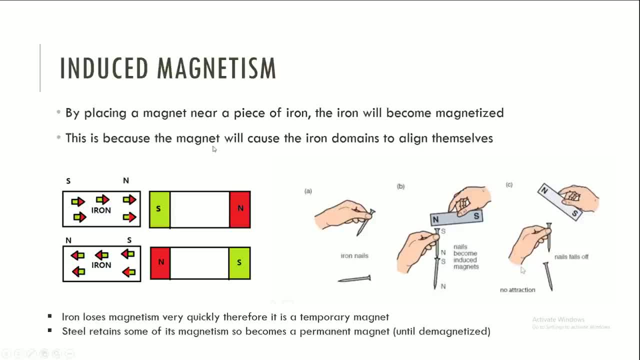 And this is because the magnet will actually cause the little domains in the iron to align themselves via the interaction of magnetic field from the magnet magnet, right? so here let's just take a look at the diagram, right? so if you put an iron right, these little domains here, the green is south pole and the red is north pole, just like the. 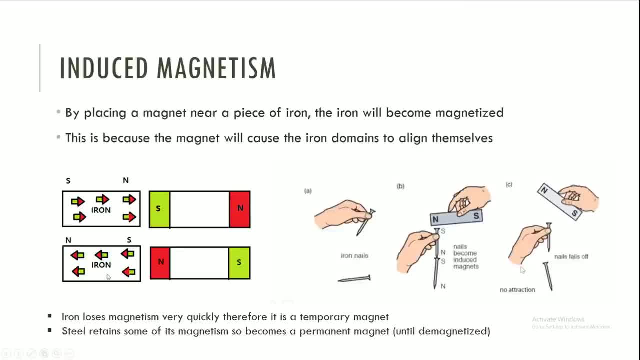 uh, the diagram below here, green south, red north, um, green south, red north, right, so you've got these little domains now, if you initially, of course, all the domains will be randomized, as i said, and iron, which is, um, you know, not a magnet, at least quite yet if you put a permanent magnet, like the one, 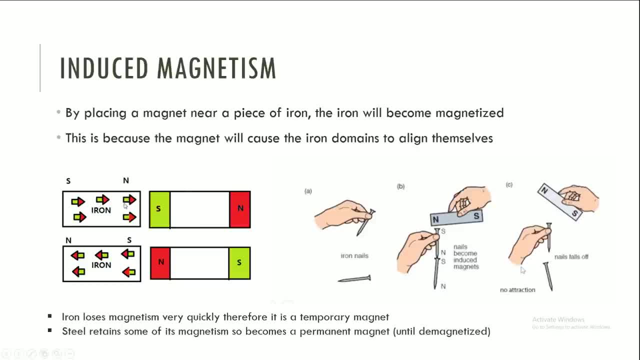 over here on the right, next to a piece of iron, these little domains will actually orientate themselves, as again, i said that opposite poles will attract each other. so if you've got a permanent magnet with a south pole right over here, then these little domains will all orientate themselves. 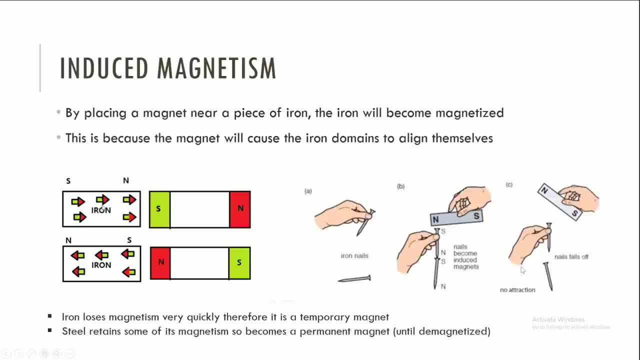 so that the north pole is attracted towards the south. so you get the alignment of the north pole towards the right and the south pole towards the left, and ultimately what that means is this iron will always get attracted to the magnet because the domains will align themselves because of the magnetic field from the permanent magnet. 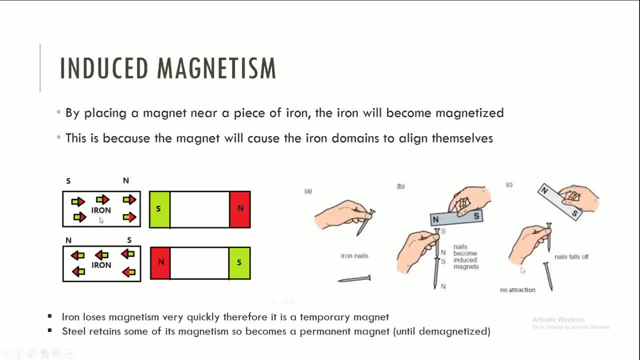 and so because the entirety, if you look at the entirety of the iron uh piece here, the north pole inherently will be towards uh, or attracted to the south pole here. so therefore you'll get that attraction um, oppositely, if you were to have it the other way. 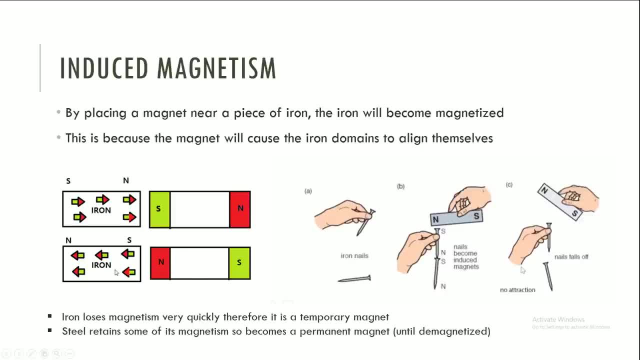 around and you have a permanent magnet with a north pole facing this way, then of course the little south poles of all the domains will align towards this end here, um, and the north pole will face away. and so, ultimately, what this permanent magnet is doing when it's near the iron? 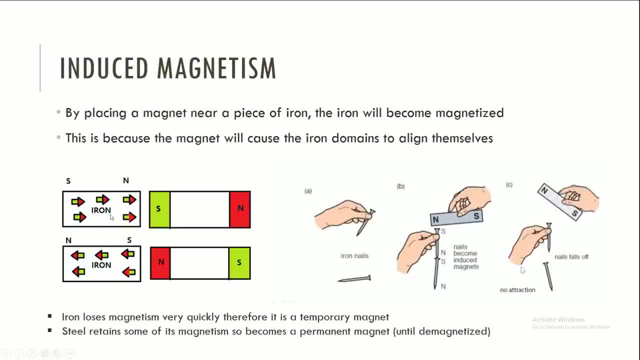 piece is magnetizing it because the domains are aligning themselves. they are turning into a magnet with a magnetic field on its own, and therefore you get this attraction happening. okay, and so if you take a look at this diagram over to the right here, this is a very practical 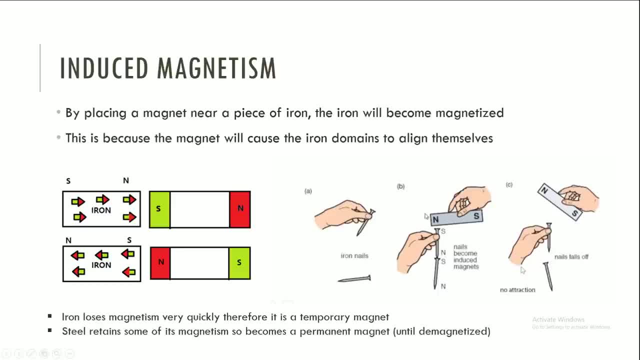 example of how induced magnetism works, right? so if you put two iron nails next to each other, you will never get them being attracted to each other. there's absolutely no force, and that's because they aren't magnets quite yet they don't have any sort of magnetism. 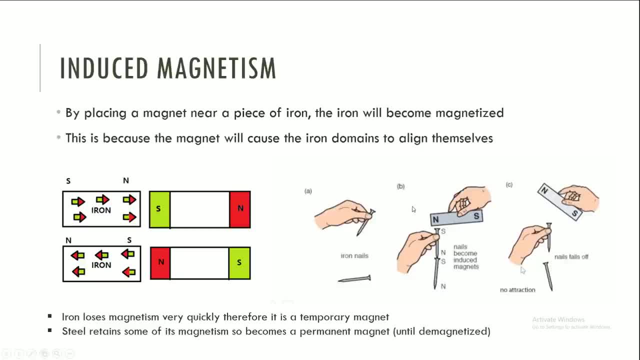 but as soon as you have some sort of magnet right- let's just say north and south pole here- then the iron will attract itself onto the magnet and, as i said, the induced magnetism will cause this top nail here. the south pole will of course be at the top, closer to the north pole, of the permanent 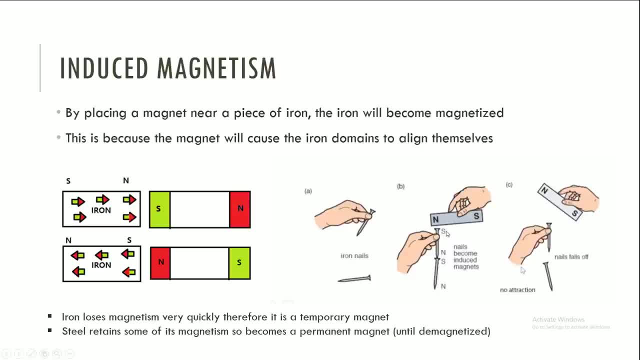 magnet because again, uh, the, the, the opposite poles will attract each other and if this top part is the south pole, then the bottom part must be the north pole and you can actually see that the second iron will actually, or the second iron nail will actually get attracted onto. 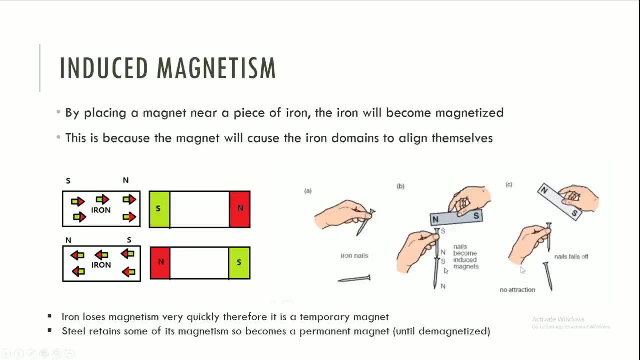 the first nail, because the first nail now has become a magnet. the first nail induces magnetism onto the second nail, and so the top part of the second nail will have a south pole and the bottom part of the second nail will have a north pole, and so therefore you get an attraction between. 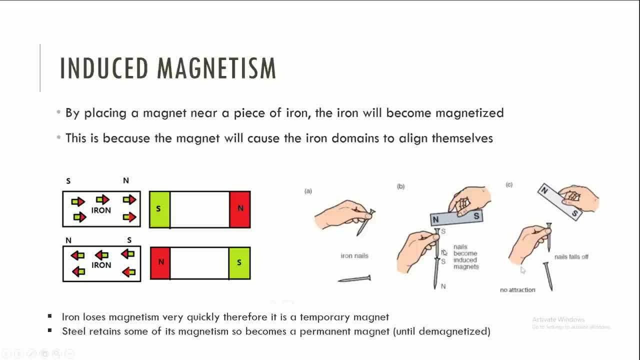 the these two nails because they are now aligned the down the way into the use of the magnet. so this learn magnetism, because they're now just magnet and, like normal magnets would, are magnets, but it's not magnets because the first nail has basically, uh, been magnetized by this top permanent magnet. okay, so, um, but if, if there was no, 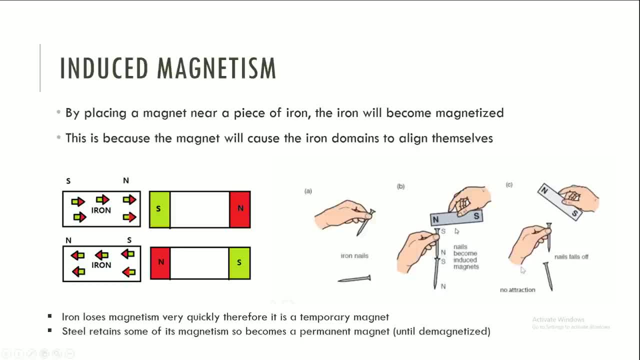 sort of induced magnetism going on there. then the two irons nails would never actually attract each other right. so essentially the idea as used is that using a permanent magnet you can magnetize or induced magnetism, domain magnets sitting inside of them. Now iron loses magnetism very, very. 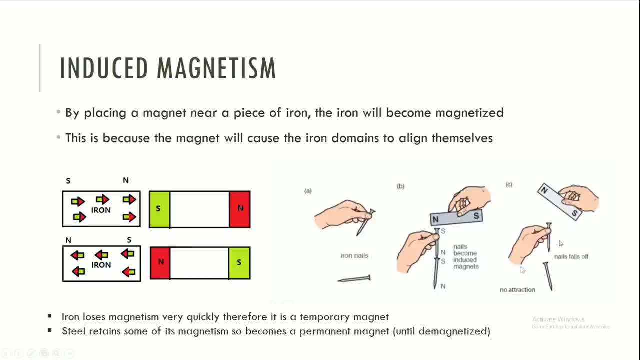 quickly. so as you, soon, as you detach the permanent magnet from the first nail, this whole thing falls apart, because both nails- well, the first nail essentially loses all of its magnetism, and the second nail also loses all of its magnetism as well as a result, and so iron as a substance loses magnetism very. 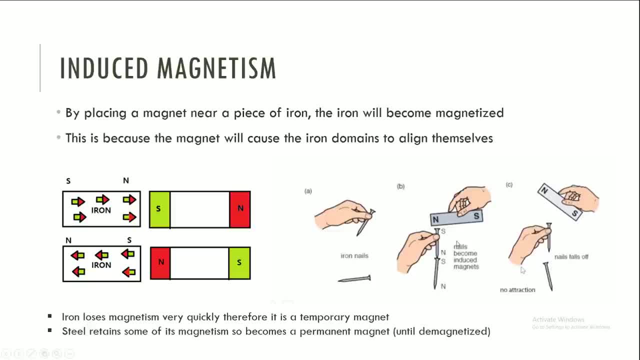 very quickly. so when it does get induced with magnetism it becomes a temporary magnet, right. however, steel, which is of course largely made of iron, but other things as well, like carbon, retains some of the magnetism without losing it completely. so once you magnetize steel, even after you sort of detach the, the 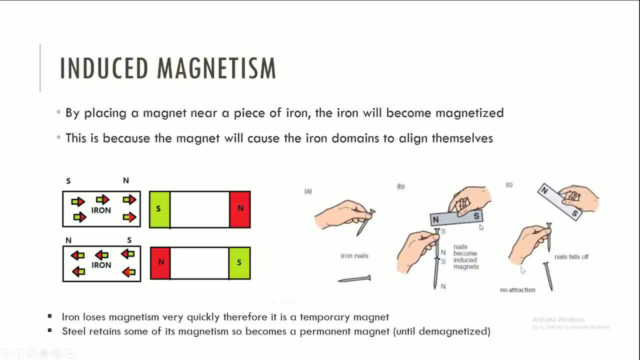 permanent magnet away from the steel, it will still have some sort of magnetism left, unless you detach the permanent magnet from the steel. it will still have some sort of magnetism left unless you demagnetize it by, you know, hammering it or whatever. we'll take a. 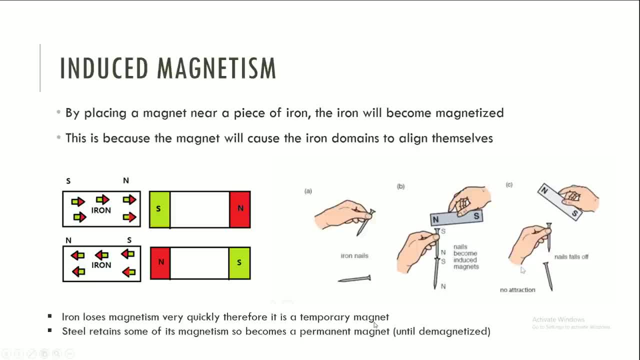 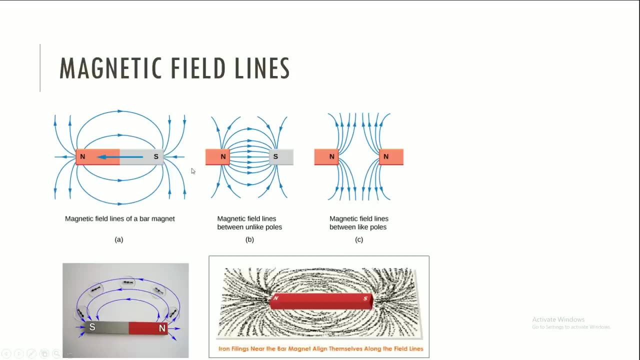 look at demagnetizing things later, but the idea is, steel can retain magnetism and become a permanent magnet, whereas iron will only be a temporary magnet because it always loses its magnetism very, very quickly, and so I suppose the the important thing here would be to understand how to draw magnetic field. 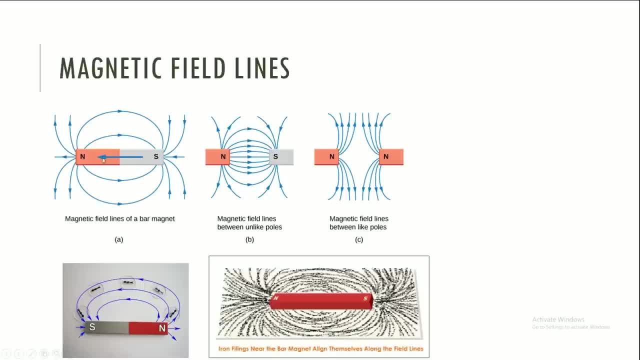 lines. I think this first image is probably the most important for you, because this bar magnet is what we are all familiar with. a bar magnet, as with any other magnet, will have a north and a south pole, and so if you draw the field lines horizontally, you'll always get the field lines going from the south to 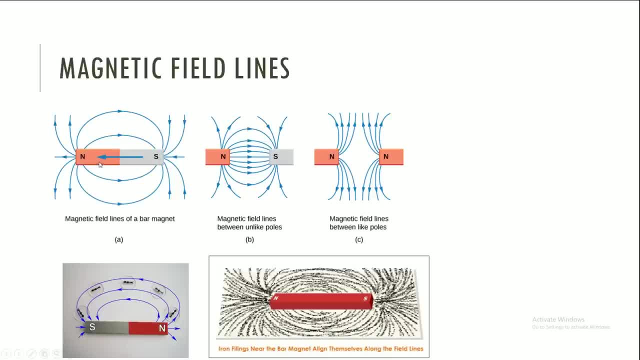 north. but if you look at the, the, the top rays, here it'll go. it'll be going from north to south, right? so this middle chunk here the rays, this middle chunk here the rays are the magnetic field lines, will always go from north to south, but the 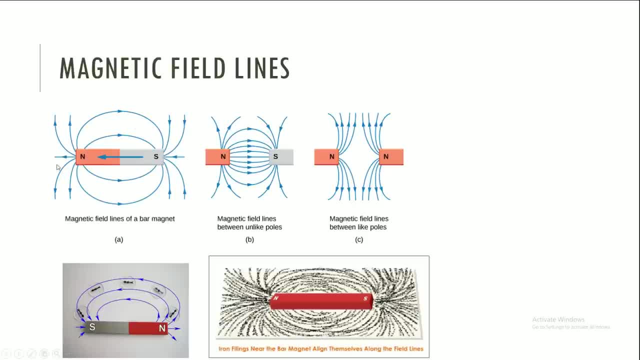 ones at the ends will always go in the direction of south to north. so just memorize how this looks, and you should always probably know how the magnetic field lines look when the poles are either attracting or repelling right. so opposite poles attract and they'll always go from north to south like this. 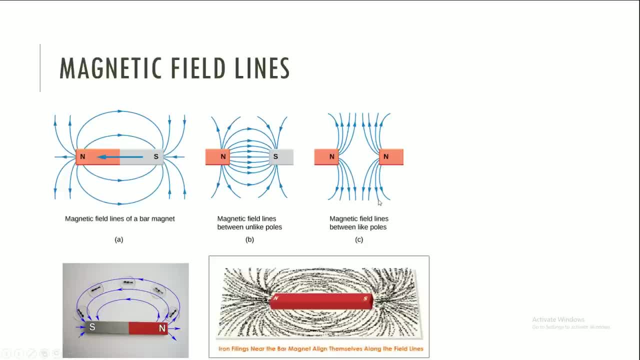 diagram here and if you're looking at two of the same poles, they're obviously going to be repelling each other and you get this sort of field line happening here. so make sure you are very comfortable drawing the south and have a look at this diagram and just memorize. 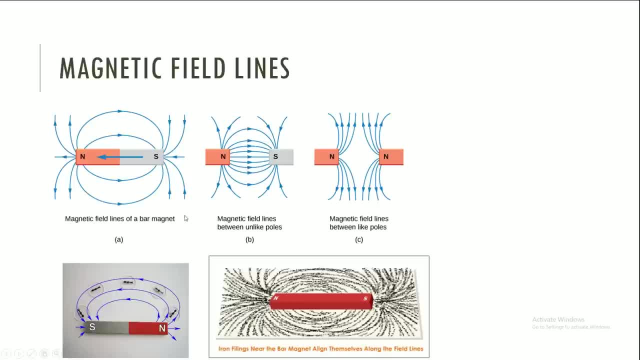 it the best that you can now, experimentally, you can actually demonstrate these magnetic field lines. first of all, you can either use a compass. so if you put like a compass in series like this around a bar magnet, the, the compass will actually point towards the direction of the field lines, like so: 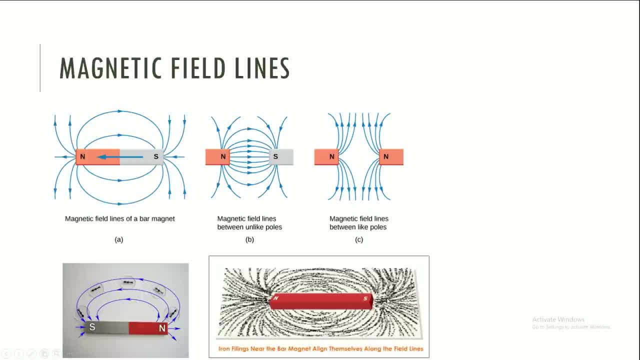 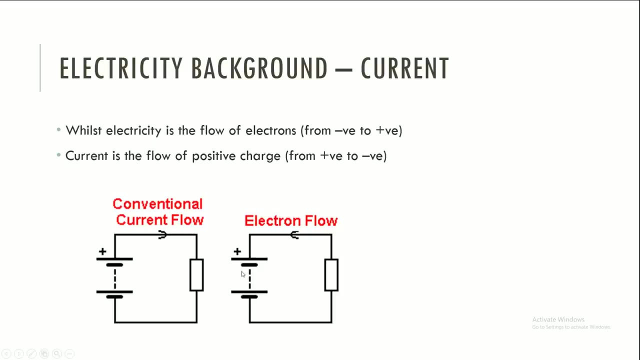 and secondly, you can also use iron sort of fillings, which are very fine iron particles, and scatter it all over the place and they will sort of align themselves along with the magnetic field lines. so this entire topic is of course electricity and magnetism, and we will combine the two in a sense and we'll do a. 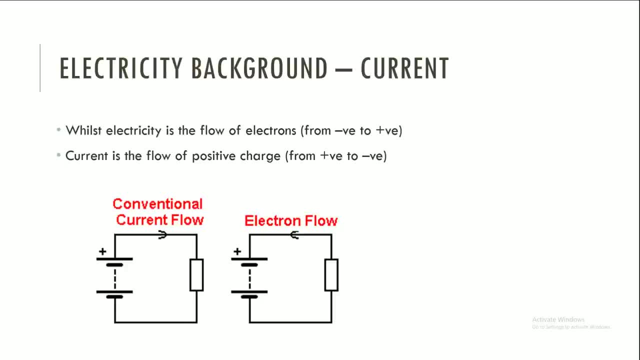 second, but some important concepts here, right? so electricity is basically the flow of electrons, and it would make sense that because of that, electrons will flow from a negative charge to a positive charge. but current is a little bit different. current is defined as the flow of a positive charge, which is from: 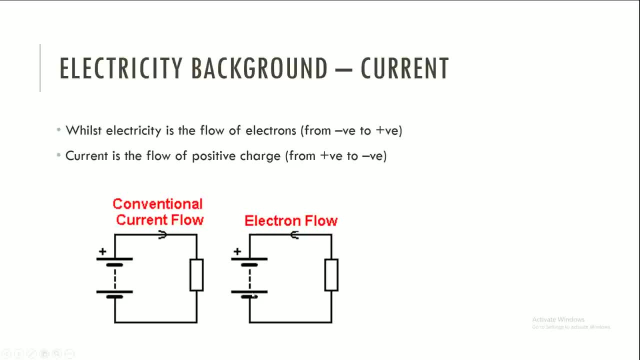 positive to negative. so if you have a look at this right diagram here, this side is negative, so you would expect that electrons to be flowing in this particular direction. but when you're thinking about current, it's actually going the opposite direction, because it's the flow of not negative but positive charge. so it's always the 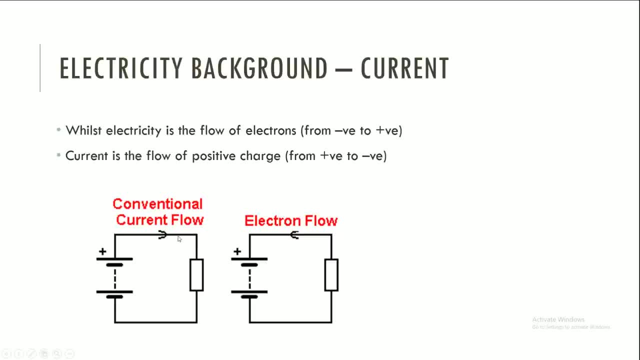 opposite way around. now, current is what we use mainly in calculations and things like that. so if they ever were to give you a direction of electron flow, then you will have to really understand that current, on the other hand, is going the other way around, and then you'll have to sort of go from there. but we will look. 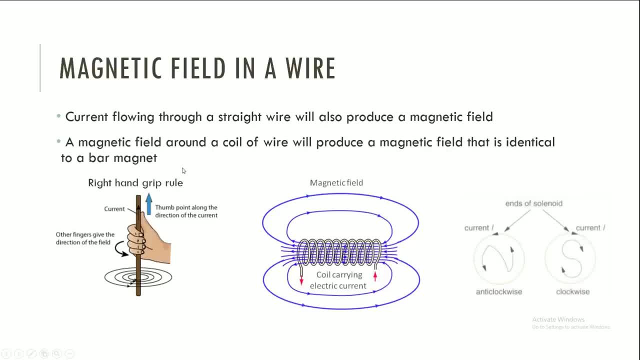 at this data for more detail afterwards as well. so while we're on the topic of electricity, of course current flowing through a wire also magically produces a magnetic field. a magnetic field around a coil of wire will produce a magnetic field that is very basically identical to what we saw of a bar magnet, right. so 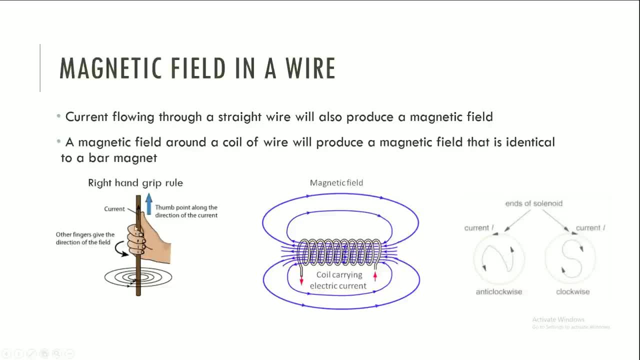 let's go through the magnetic field, through a straight wire on the left hand again is going upwards, but the flow of electricity or the flow of electrons is going downwards. but anyway, current we are going to suggest that it's going up, and so if we point our thumb right, this is called the right-hand grip. pull like. 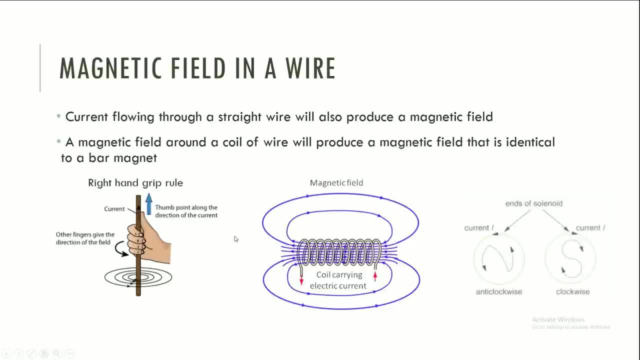 as the diagram shows here, point your thumb towards the direction of the current, and the fingers which wrap around the wire will give the direction of the magnetic field that the wire produces. now, if you were to get a long wire and coil it up like this diagram in the middle here, then it will produce the 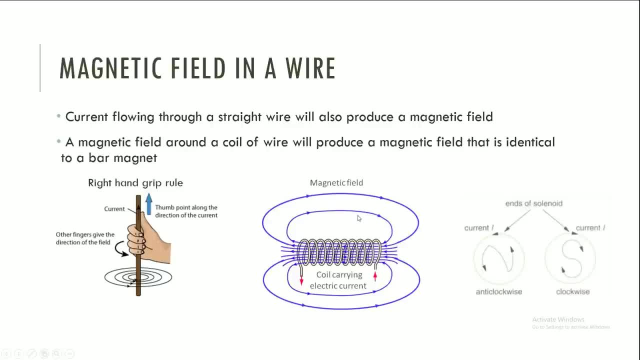 magnetic field, just like a bar magnet. so again, as we took a look at before, the horizontal lines in the middle is going from left to right here, oh sorry, right to left, going in that direction. and so remember, in a bar magnet it's, it's, it goes from the south to north pole. so if you were 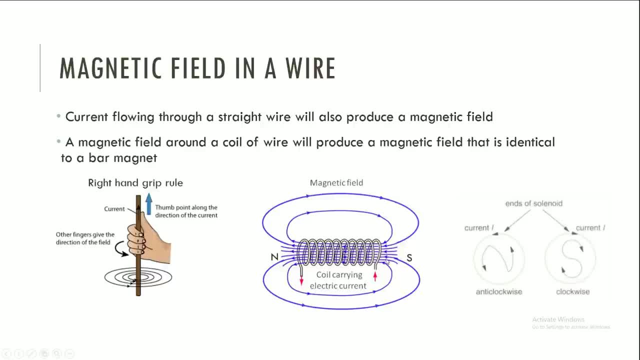 to you take a look at the poles of the magnetic field that this thing produces, then you can sort of judge by the field lines that this side here to the right is the south pole and this side here is the north pole. but even if I didn't give you these field lines and the direction of field lines, 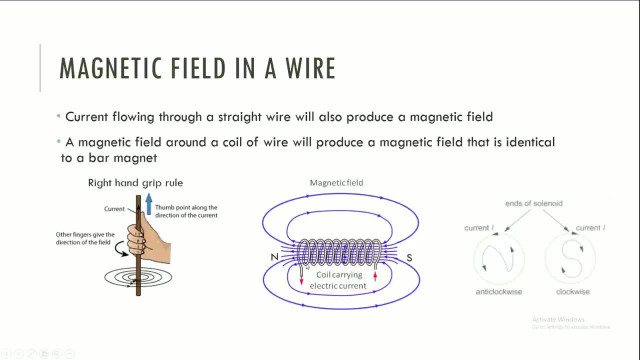 you can actually tell which side will be the north and which side will be the south pole just by looking at the direction of current in the ends of the coils. so if you take a look at this left hand side here and imagine if you are looking at it from a head-on, straight-on perspective, you can 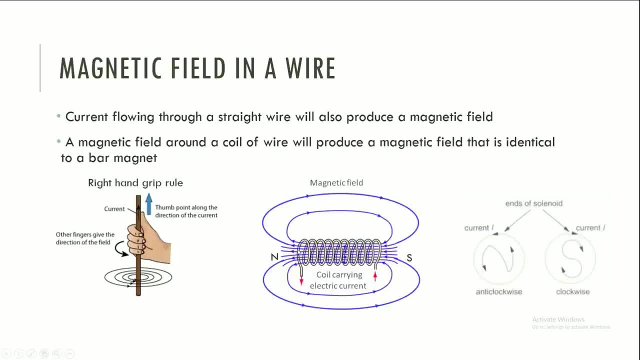 see that the electricity is actually going in an anti-clockwise direction, or current is flowing anti-clockwise in the wire. so take a look at this left diagram here. you can see that it goes from the Re-fine. you can see that it goes from the re-fine to the red line and actually 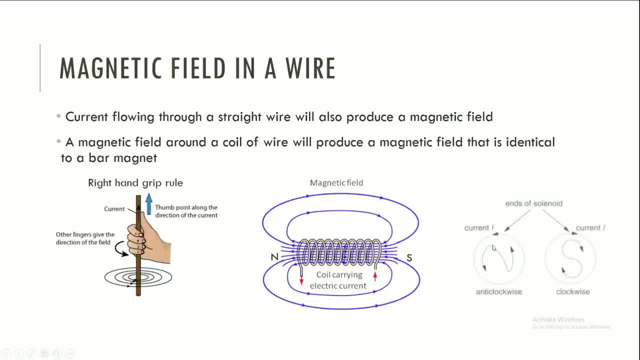 gets to that directly, straight way. it goes from here. it goes to this thirst line, to the next line, and then you can see. This is the sort of direction of the current that you'll see in the end of the coil on the left-hand side here. 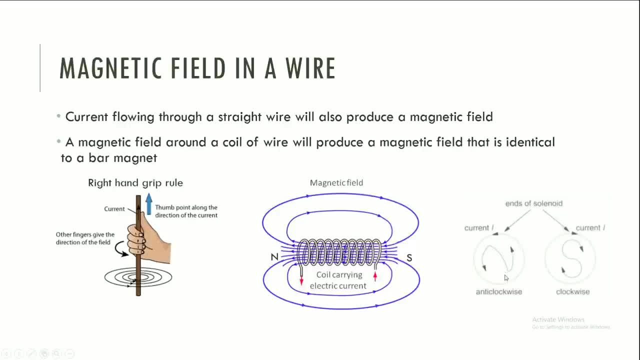 And so an easy way to memorize that would be that it makes the shape of an N here, and therefore north. On the other hand, if you look at the right-hand side of this coil of wire, you will actually see that the current is flowing clockwise. 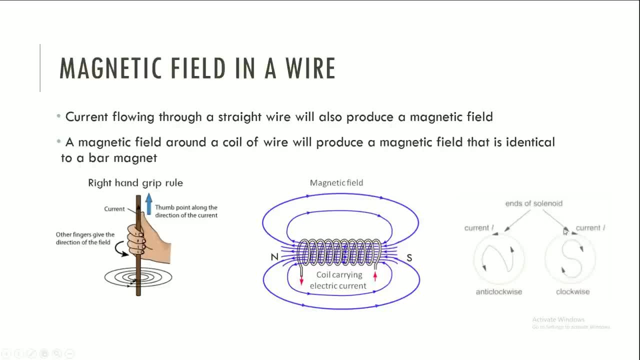 And so if you take a look and see the shape that it makes, it's sort of like an S shape here, right, And so that would suggest that it is the south pole in that end. So that is a pretty handy way of knowing the north and south poles created by the magnetic fields of a coil of wire carrying a current in a certain direction. 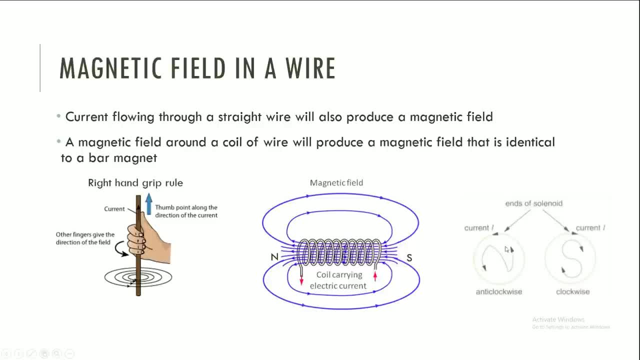 What's really important to note here is that, again, the north and south poles created by the coil of wire is solely dictated by the direction of the current right. So if you look at one end and it's going anticlockwise, then again that's the north pole. 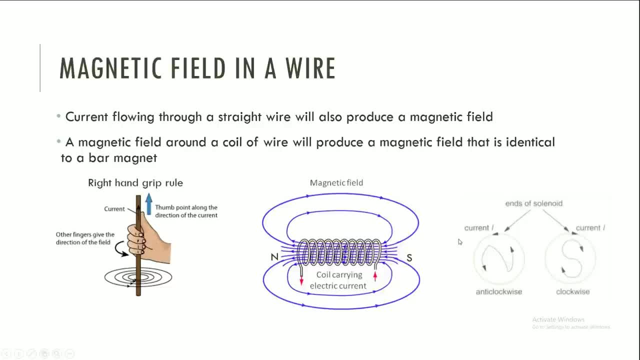 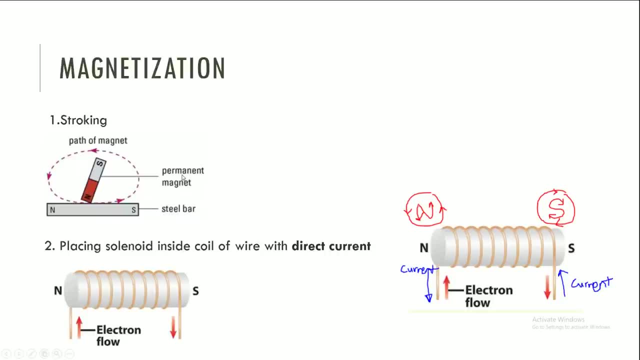 If it's going clockwise, it's the south pole. So we will take a look at that in this section here. But first of all, magnetization: If you want to magnetize a piece of wire, you want to magnetize a piece of wire. 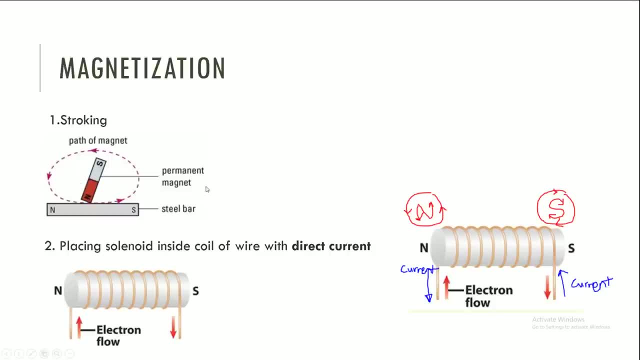 If you want to magnetize a piece of steel or something like that, one way of approaching that would be by stroking it with a permanent magnet in a sort of circular direction here, so that you are overall sort of nicely aligning all the domains in the steel bar so as to induce permanent magnetism in the steel bar. 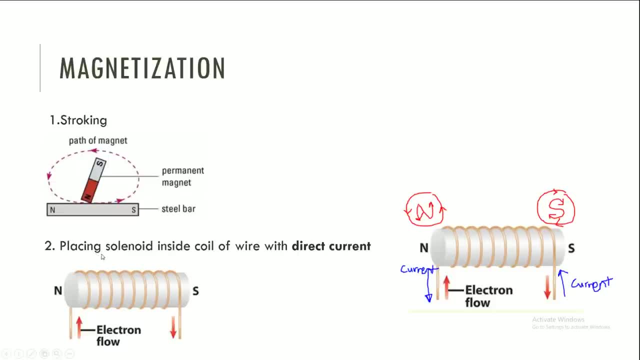 But, as I was saying before, electricity-wise you can also magnetize metal or steel or iron or whatever by placing a solenoid. But, as I was saying before, electricity-wise you can also magnetize metal or steel or iron or whatever by placing a solenoid, which is basically metal, inside a coil of wire, like the setup here with direct current. 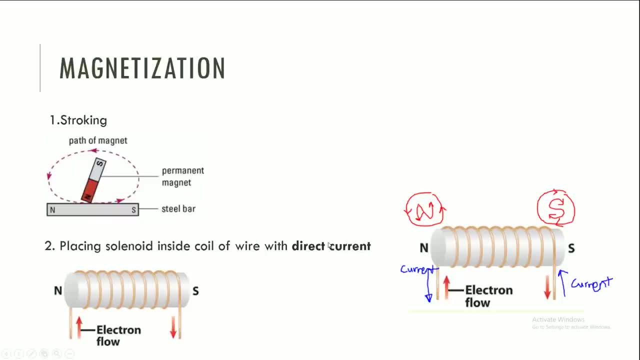 And direct current means that the current is always going in one direction. okay, Alternating current is when the current is changing directions all the time, constantly, But direct current is in one direction all the time. And that's obviously very important because if you want to magnetize a bar of steel or whatever, using the 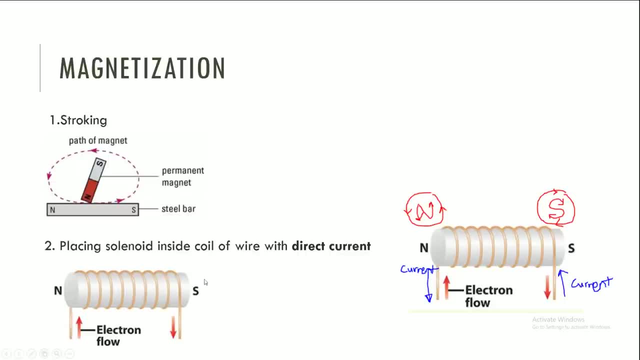 magnetic fields. of a coil wire, which we talked about before, then it needs to have a consistent north and south pole, Otherwise the magnet will, or the steel will, never get magnetized, and that's why direct current is really important here. 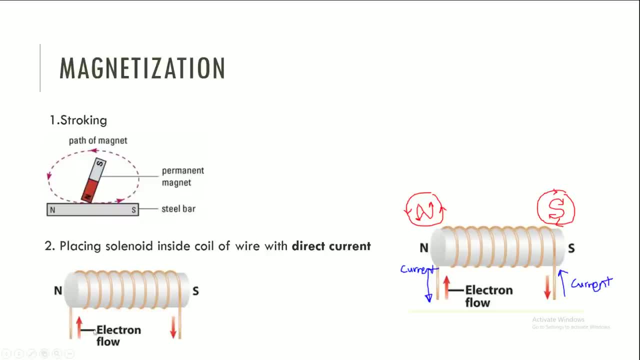 And so the electron flow is going upwards, but again current will be going the opposite direction. So if you take a look at this particular diagram here I've labeled current going down, and if you use the tip I told you before, we can see that in this end here it's going anticlockwise. 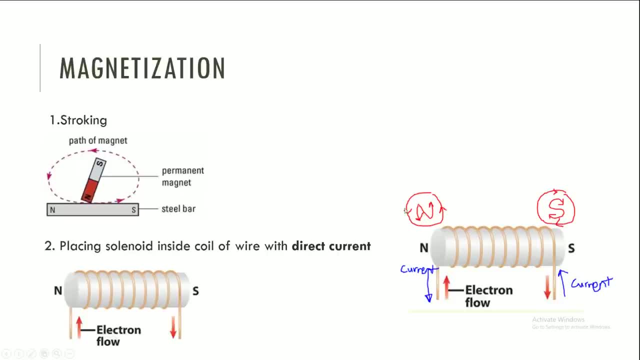 On this end. here it's going clockwise. so therefore you have the north pole on the left-hand side and the south pole on the right-hand side, And that magnetic field produced by the coil will inherently induce magnetism in the metal inside the coil, which is what we call a solenoid. 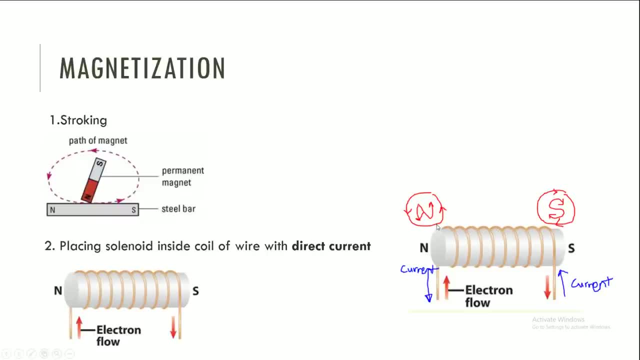 And this setup is essentially what the theory behind this is, And this setup is essentially what electromagnetism is right. Electromagnetism is basically generating magnetism by electricity, which is what we're doing here, And this is actually quite useful and, for example, when you're moving scrap metals and things like that in those metal scrap yards. 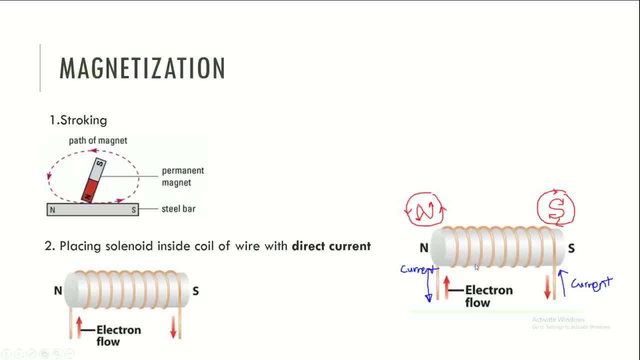 they use this theory And so as soon as you turn off the electricity, then the entire setup loses magnetism and therefore sort of drops the scrap. But if you want to pick it up again, you simply turn it off And you can just turn on the electricity and it generates the magnetism and it, you know, picks up the scrap metals and you can sort of transport it and things like that. 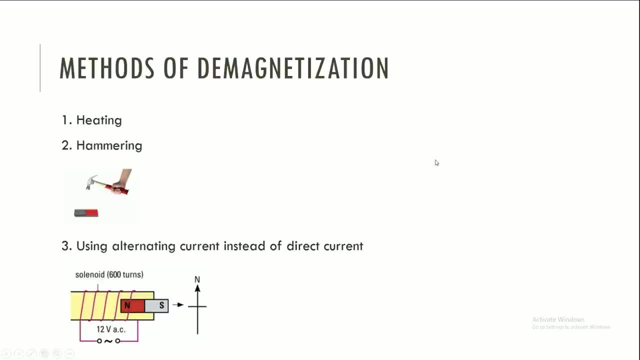 So that's quite handy. So if we took a look at the ideas of magnetizing something, you can also demagnetize something. And if you want to demagnetize a permanent magnet, you can either heat it like crazy and all the little domains will start to, you know, start misaligning itself.